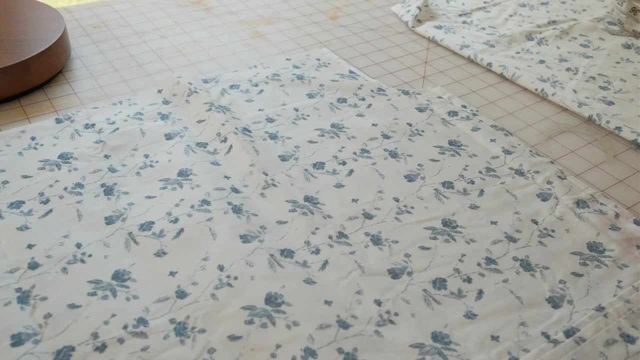 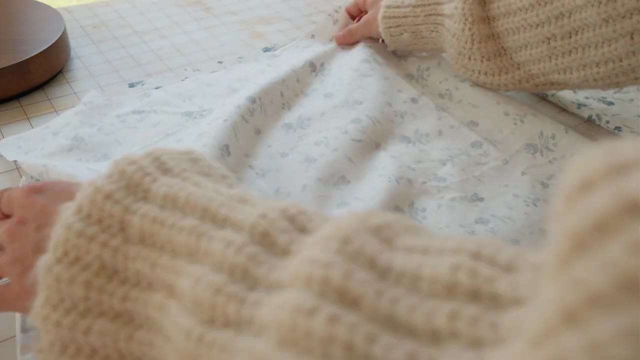 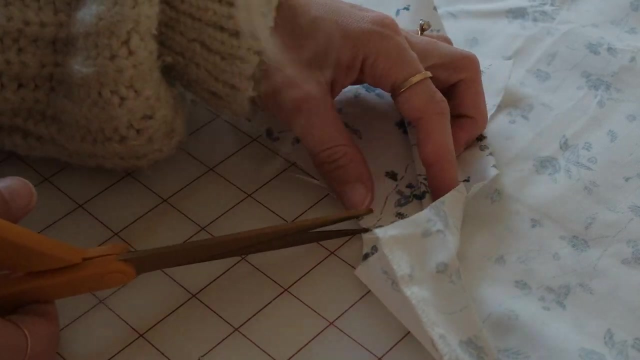 pillowcase, Make sure it's opposite to where the fold is so that when you open the pillowcase you'll have two armholes. Turn your pillowcase wrong side out and around the curved edges of the armhole and at the corner where the seam is. you want to just make a little notch and you're going to fold over. 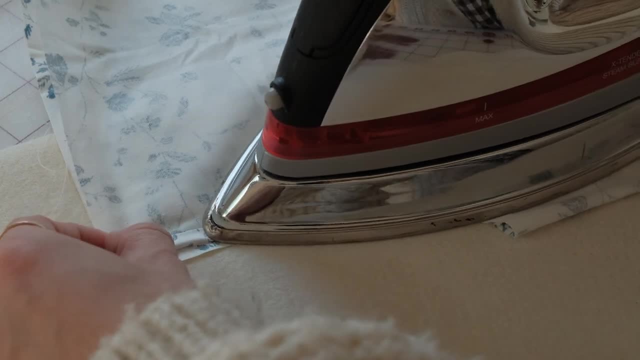 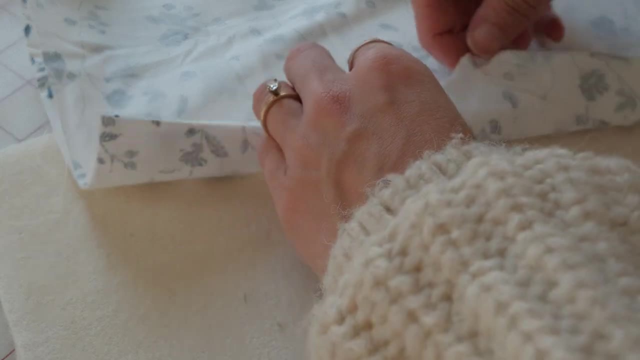 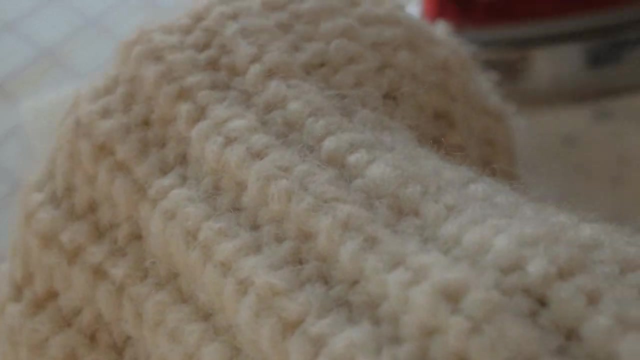 the fabric about an eighth to a quarter of an inch all the way around the armhole. It's a little tricky on the curved edges. that's why we made these notches, Iron it, and then you're going to fold it once more to enclose this open edge, and this is where you'll create your seam. 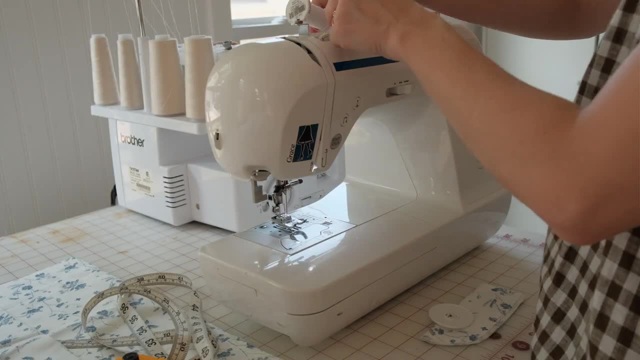 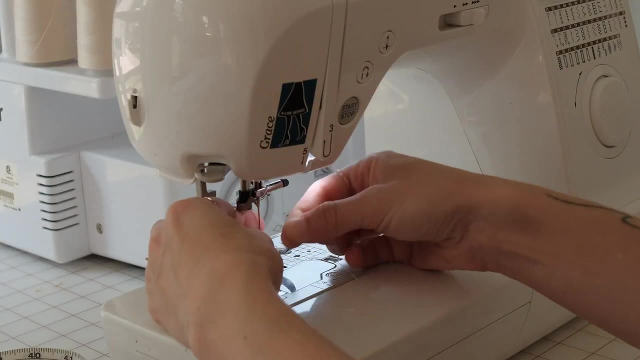 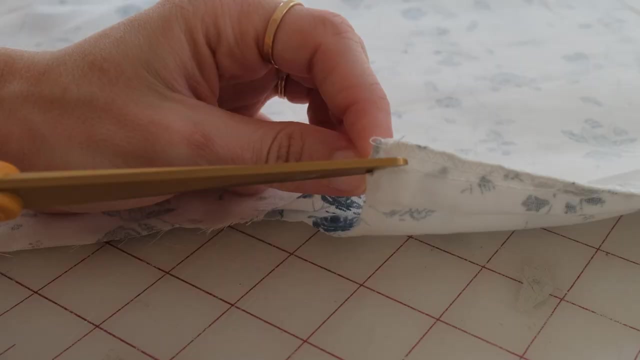 You can make as many notches as you need so that the armhole can kind of follow that curve easily. Make sure you change out your thread to match the pillowcase and sew along the edge of the arm opening. Repeat this for the other armhole. 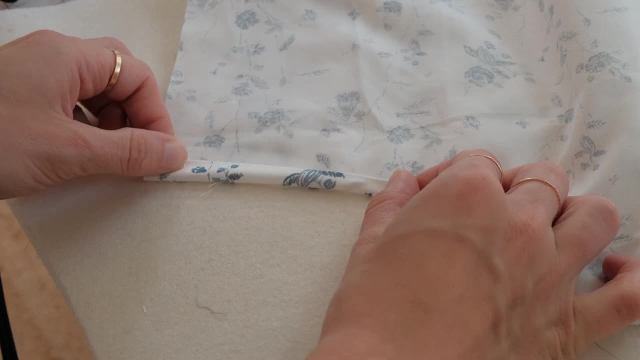 1,, 2,, 3,, 4,, 5,, 6,, 7,, 8,, 9,, 10,, 11,, 12,, 13,, 14,, 15,, 16,, 17,, 18,, 19,, 19, 20.. 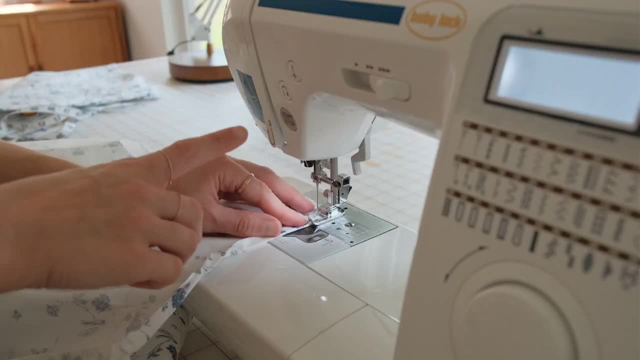 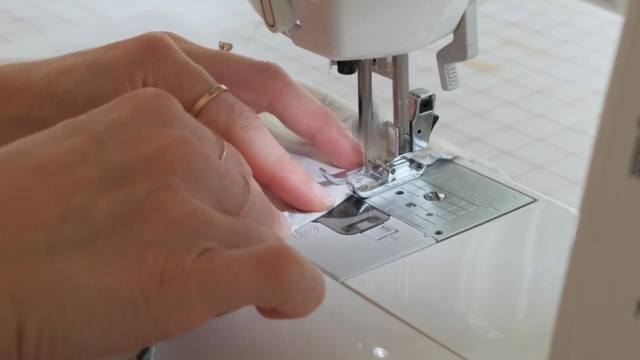 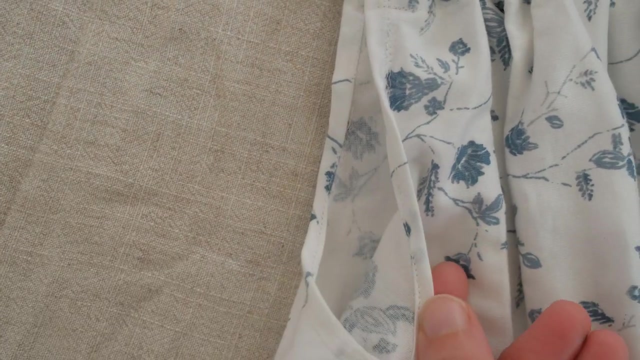 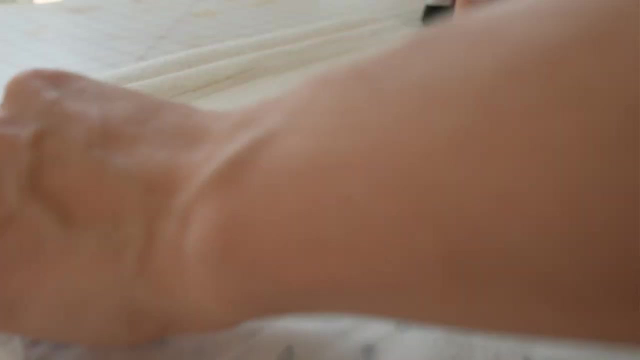 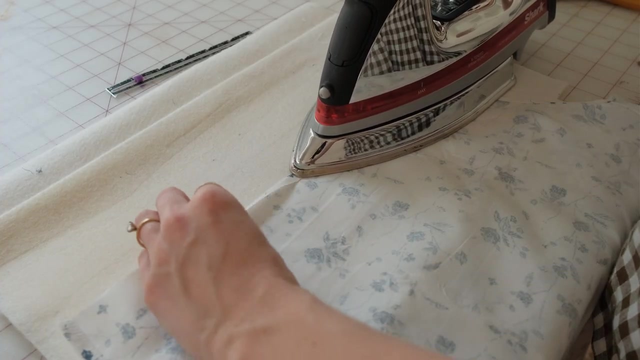 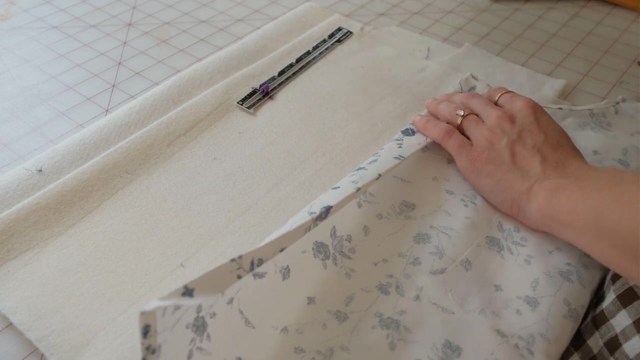 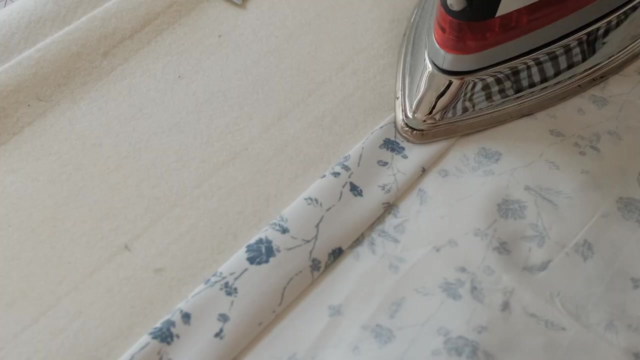 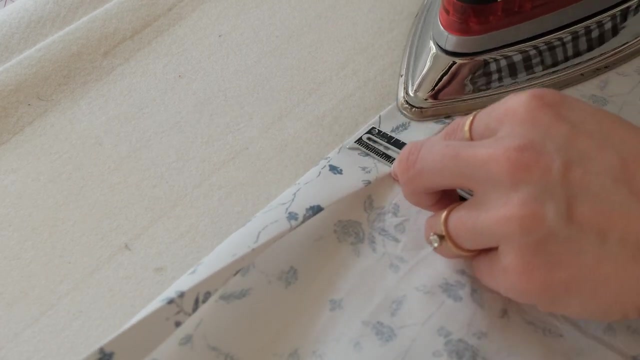 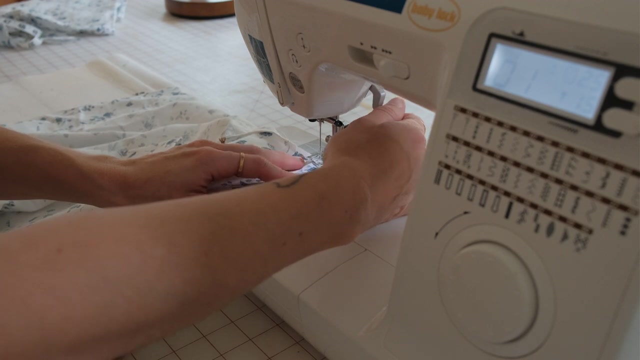 Keep going. And now, at the top of the pillowcase where you cut across, you want to the top half an inch and then press this in place and then fold it once more an inch to create a channel for the drawstring to go through From the right side facing up. do a top stitch across, making the channel and you can make. 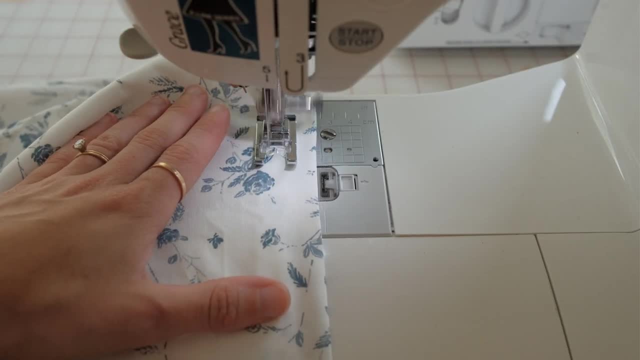 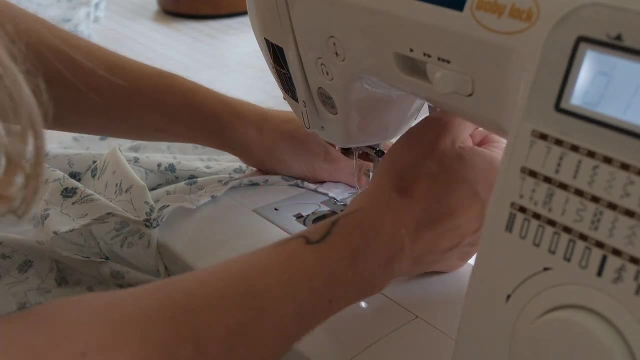 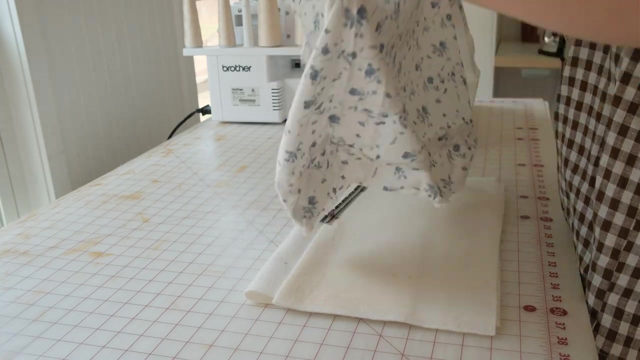 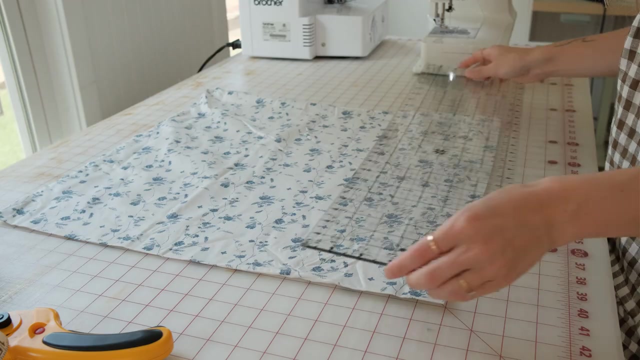 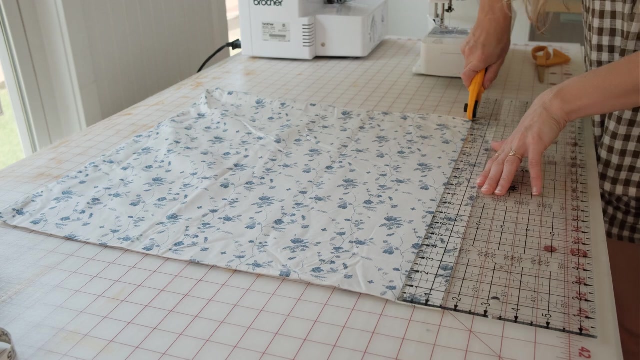 sure you're sewing right along the edge by using a little measurement along the way. Turn your dress right side out, and now we're going to make the straps for the drawstring opening. Use your remaining pillowcase fabric and cut an inch and a half by 20 inch piece. 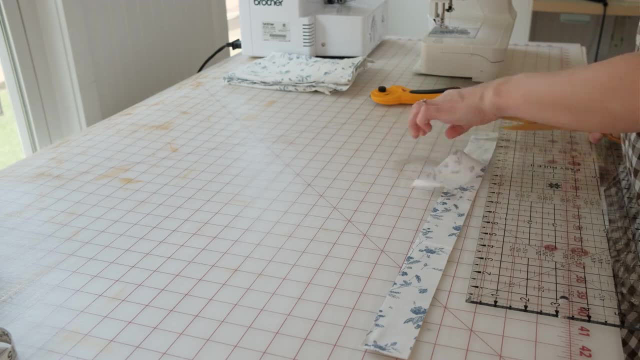 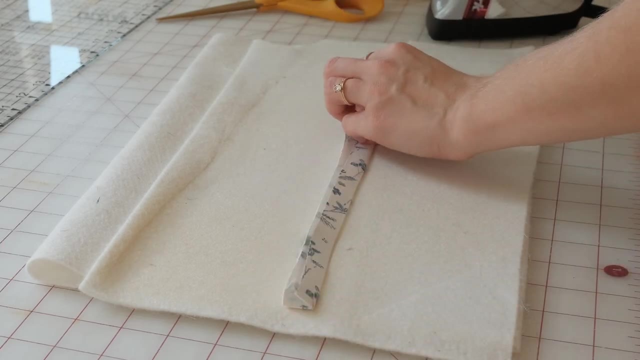 You're going to want two of these, so since the pillowcase is already folded in half, you can just cut this in half. Now you're going to fold the strap into thirds and sew along the side, So this is how you're going to do it. 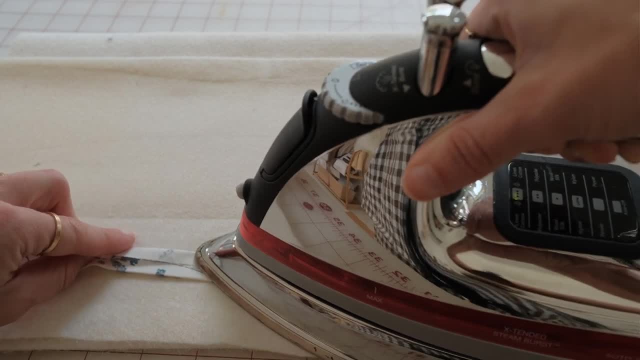 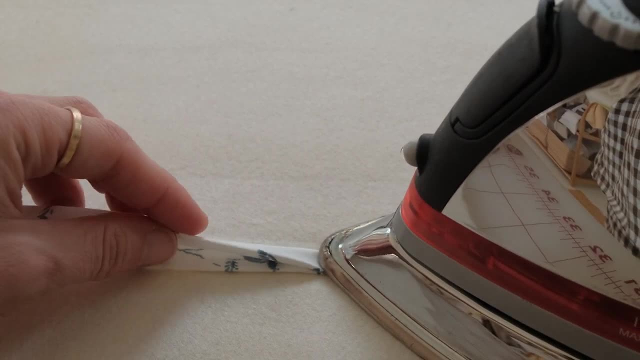 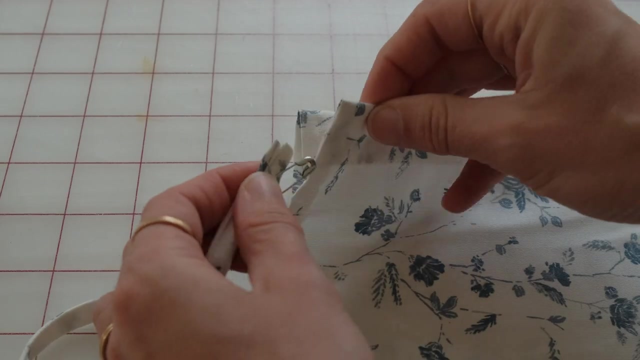 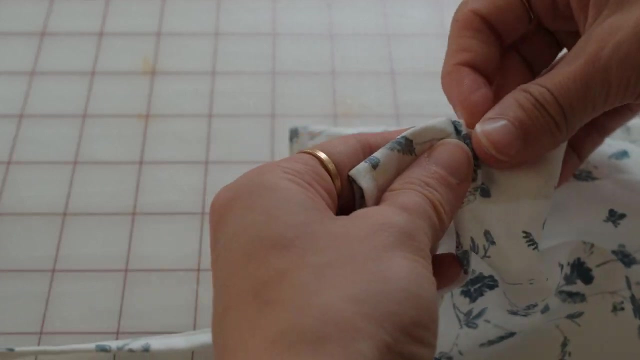 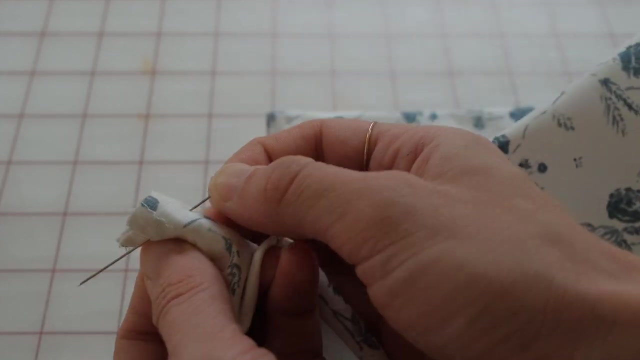 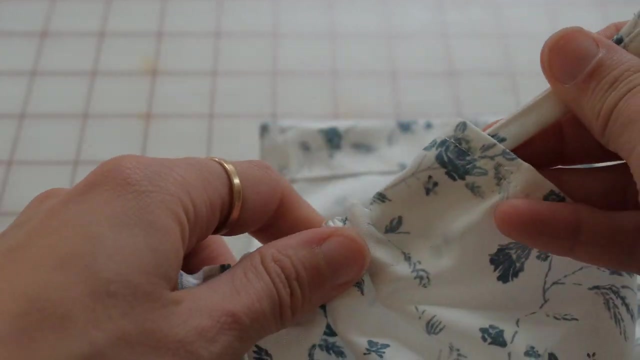 Add a safety pin to the end of your strap and start weeding it through the channel. When the end of the strap reaches the end of the channel, you can pin it in place to make sure it doesn't get lost in the channel. When you reach the end, cinch up and gather this channel together, and this is when you 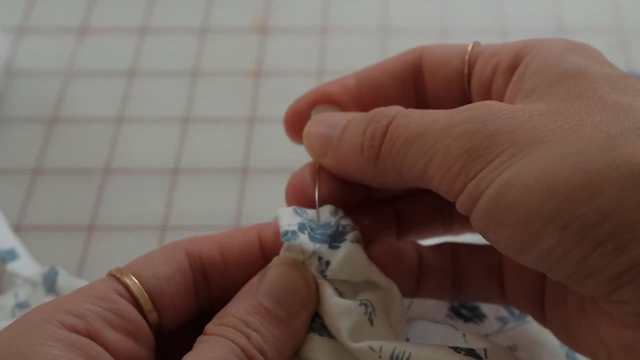 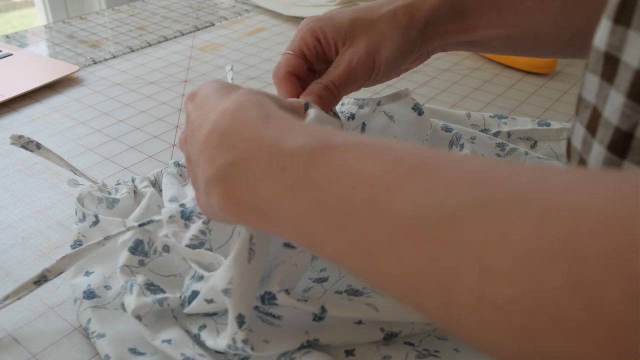 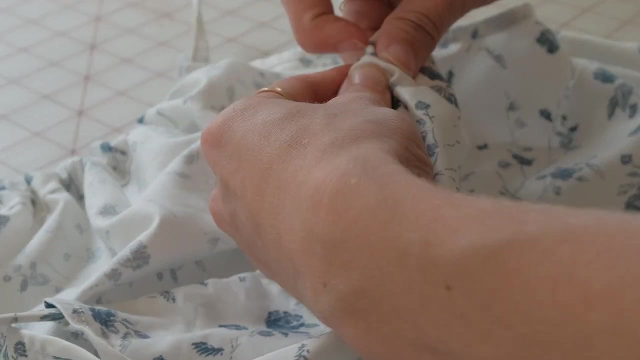 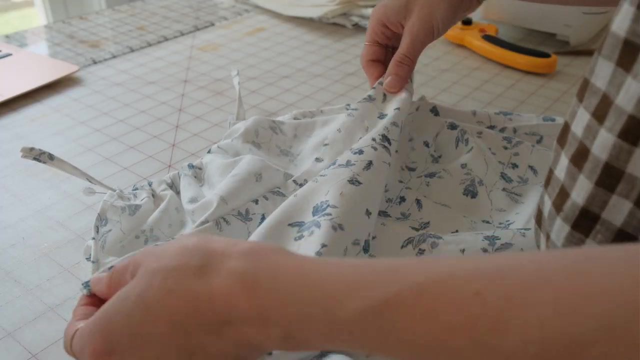 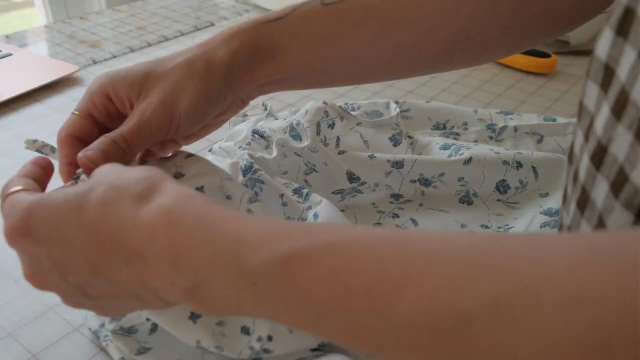 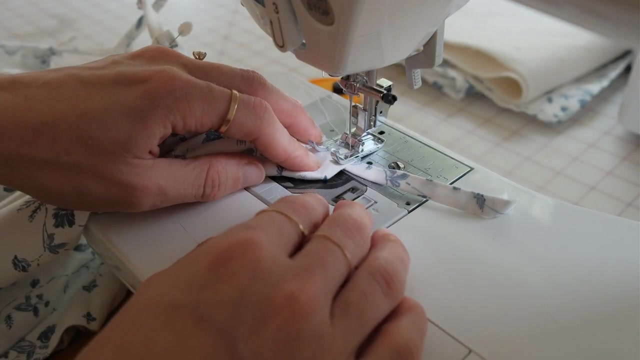 want it to measure the chest measurement of your daughter. Once it is the correct width, you can pin it in place And you want to sew a top stitch across the stitches that are already at the end, and this is going to just keep the top stitch from sticking out. 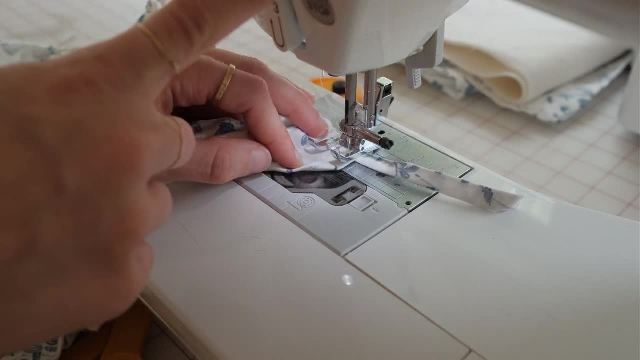 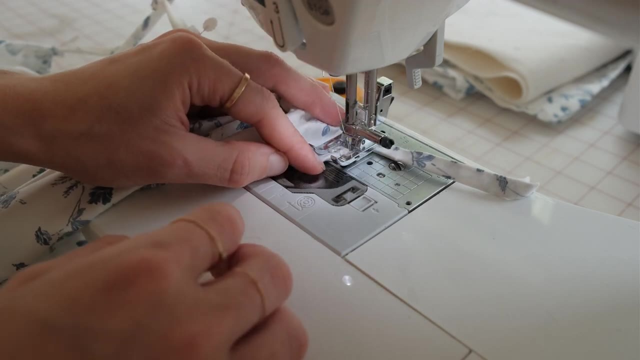 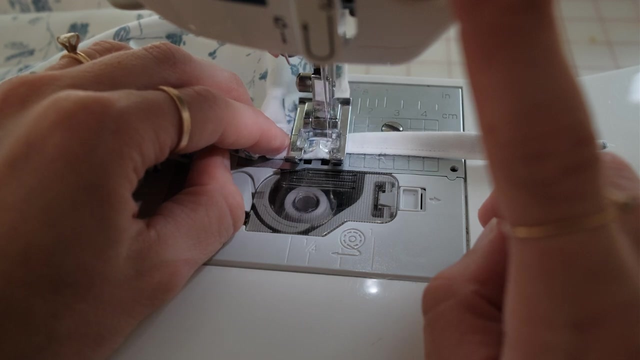 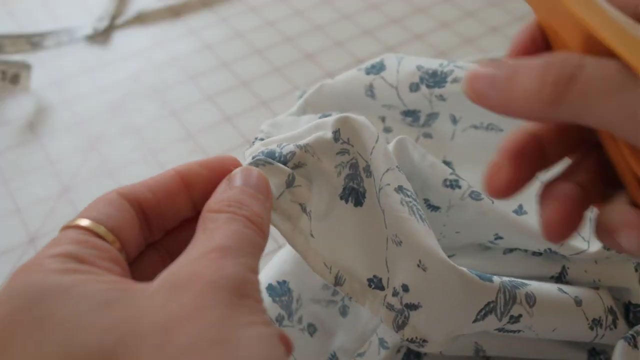 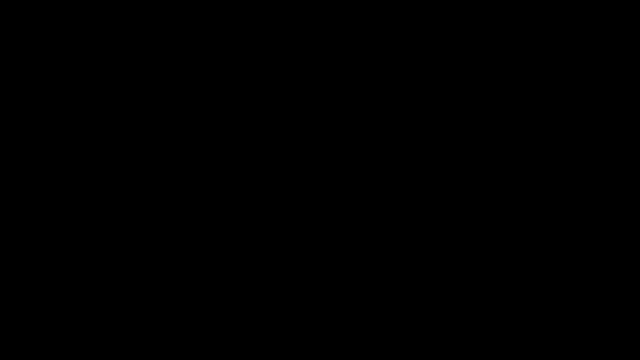 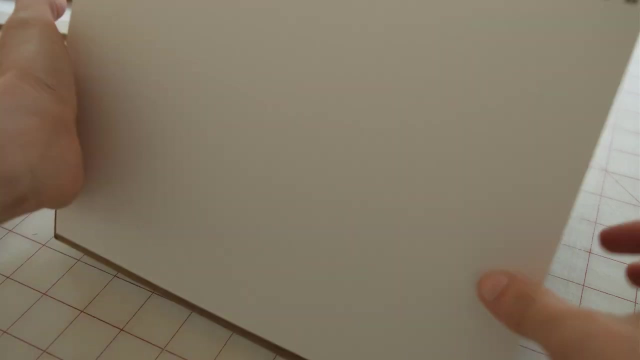 Do the same thing for the back piece, and then you can tie your straps together and your dress is finished. For the second way to make a pillowcase tutorial, this one is just as easy. it has a few more steps, but it doesn't mean it's any harder. 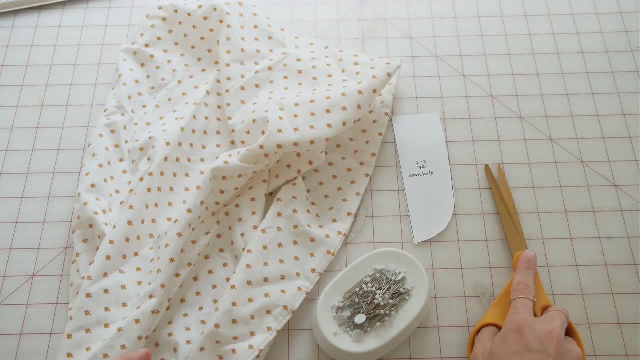 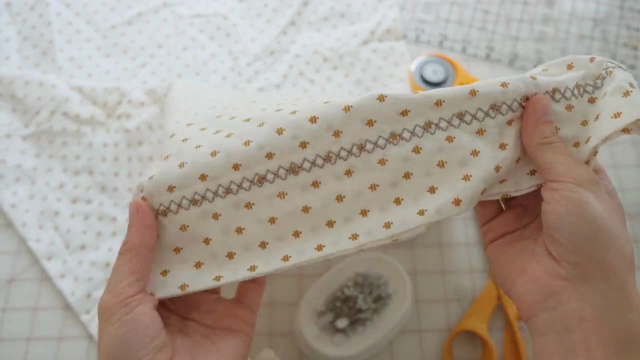 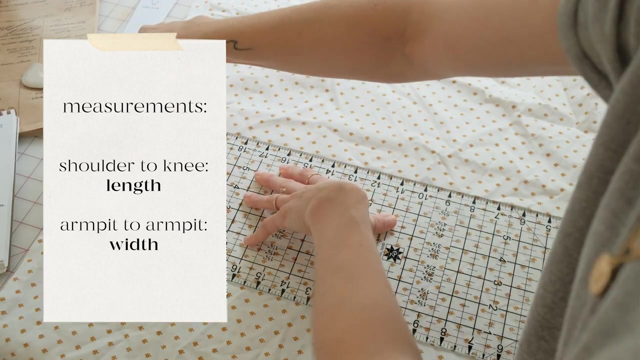 I think it's nice to have a different method and what you're going to do is the same steps apply from the first one. You're going to measure out your pillowcase and measure from the bottom hem, Measure from your child's shoulder to wherever you want it to land, because we'll be cutting. 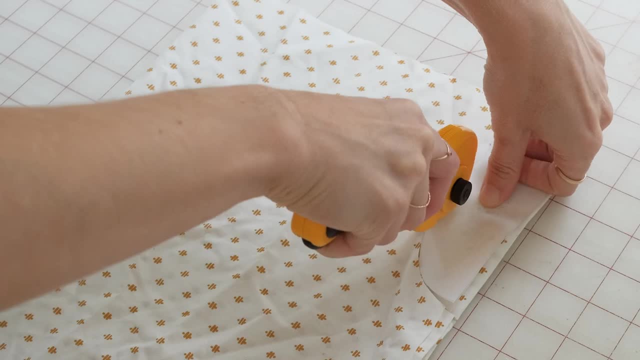 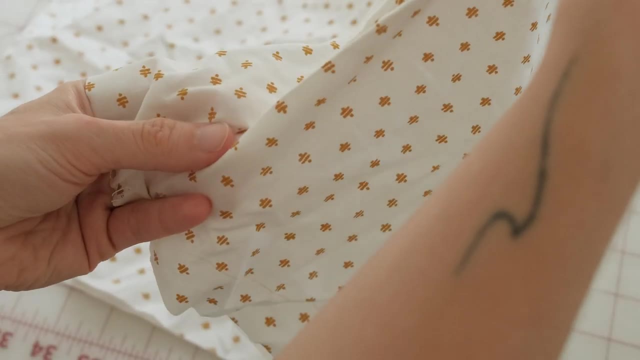 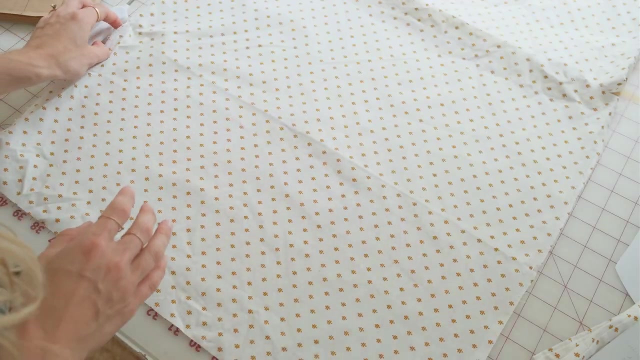 off a few inches with the sleeves, Then you're going to open it up with the remaining pillowcase or a coordinating fabric. You're going to seam, rip the edges to create a larger piece of fabric, and I measured roughly around the opening of the armhole pattern that I'm using and doubled this and then added: 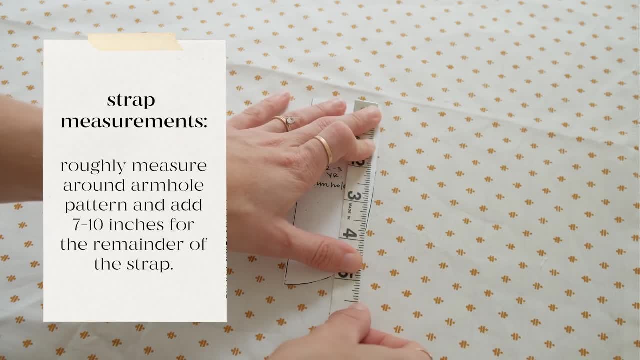 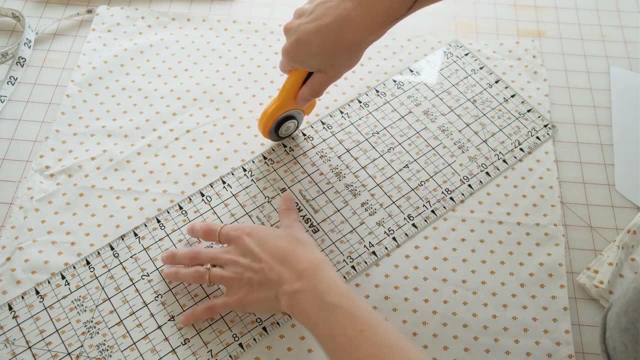 about seven inches, And this is going to be the strap. I'm cutting this on the bias, which means 45 degrees across the fabric, and the reason I'm doing this is because it's stretchy and it's going to allow the fabric to curve nicely. 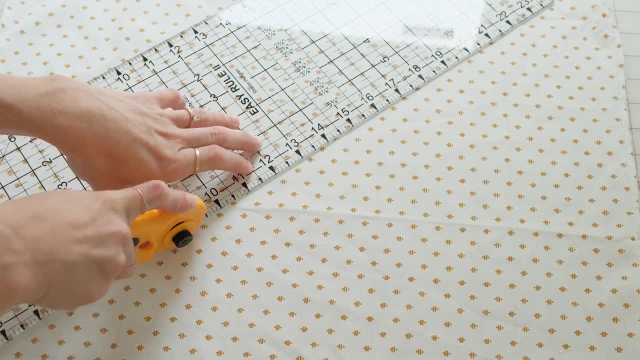 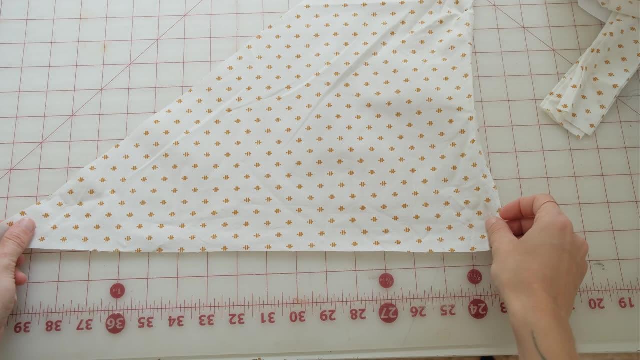 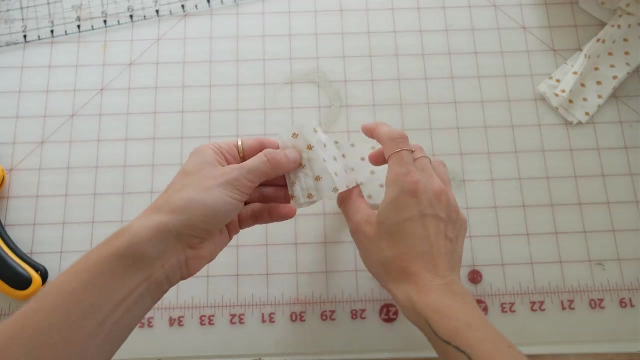 around the armholes. The same bust measurement from armpit to armpit. You're going to take that measurement and cut a two inch strip. You're going to cut two of these. This is for the front, This is for the back. 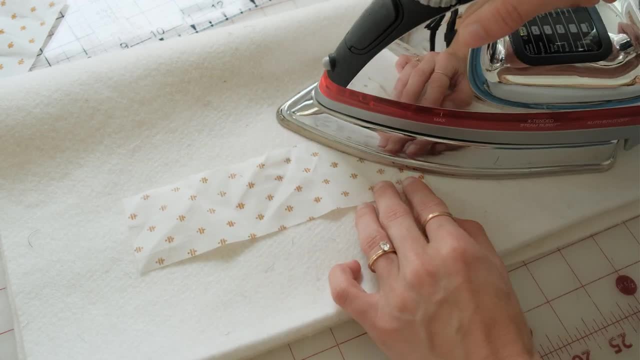 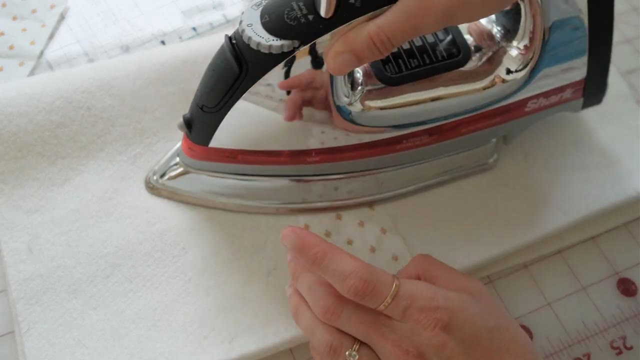 You want to fold over your fabric pieces, making sure you're folding in the end and then folding it in thirds. It's going to create this bias tape that you're going to use around the armholes, and you're going to do the same method for the chest piece. 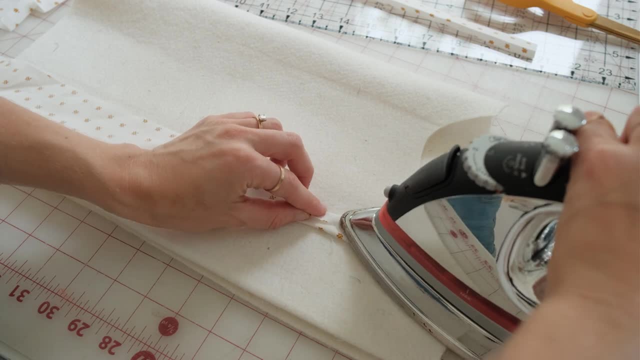 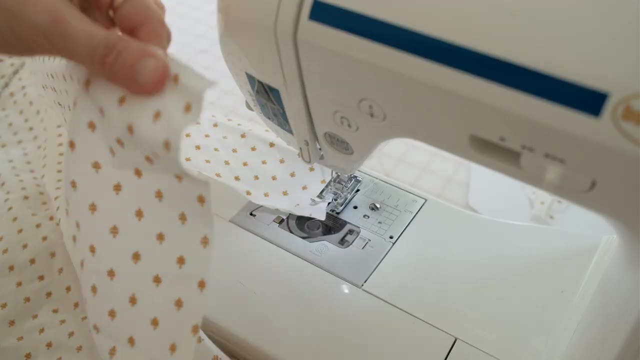 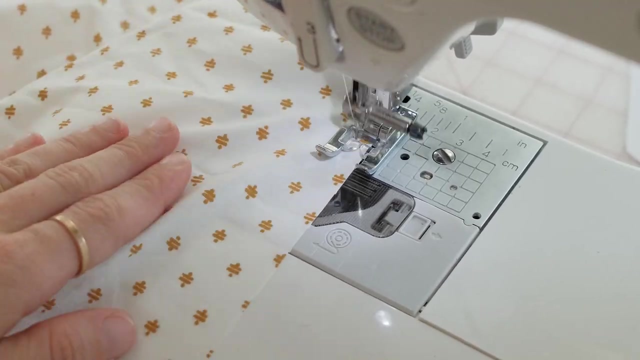 Give it a good iron and then you can move on to the next steps. We're going to do a gather stitch, so you're going to move the stitch length on your sewing machine As far as it can go. that is level five, and I'm going to sew across the top of the front. 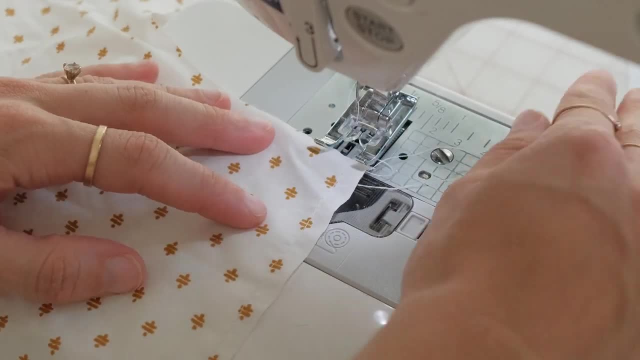 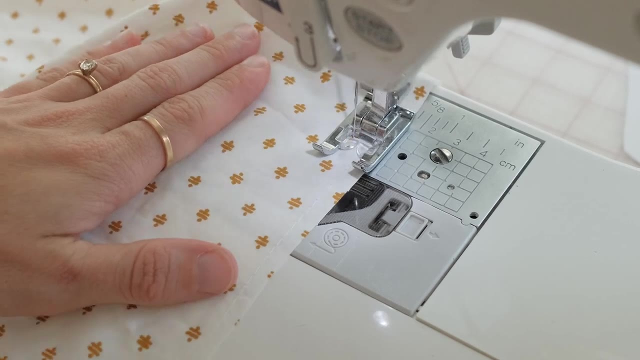 and the back with two rows. This is going to create leverage for me to hold on to the bobbin and gather the front and the back to the same measurement of the armpit front piece, And you're going to do the same thing for the back. 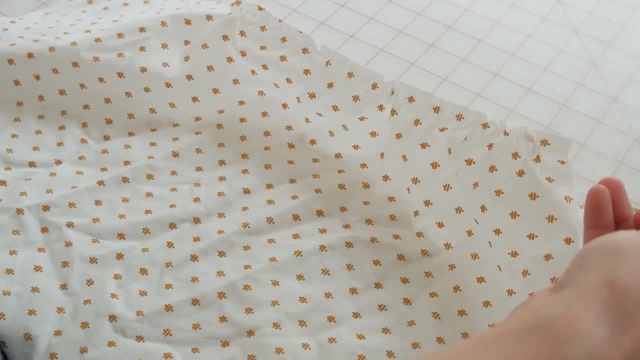 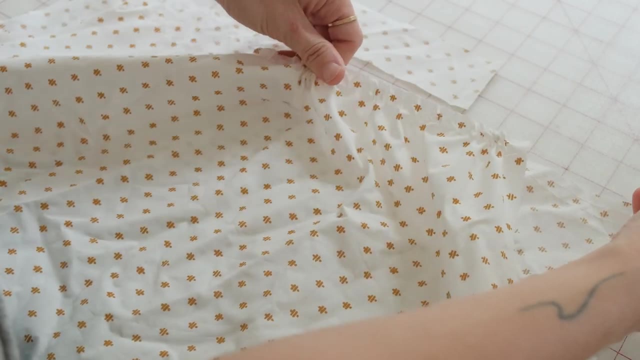 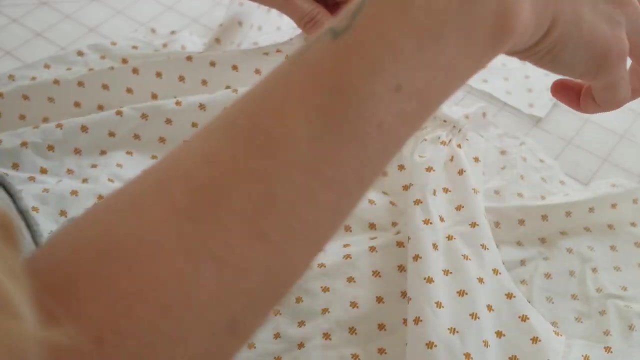 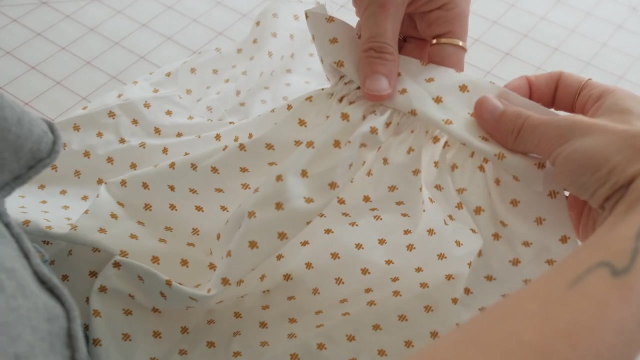 Once you have it all gathered up, you can lay out your rectangle that you cut earlier in front of you and just move around the gathers until it's the same width as the piece in front of you With the right sides facing together. pin your front rectangle to the front side of. 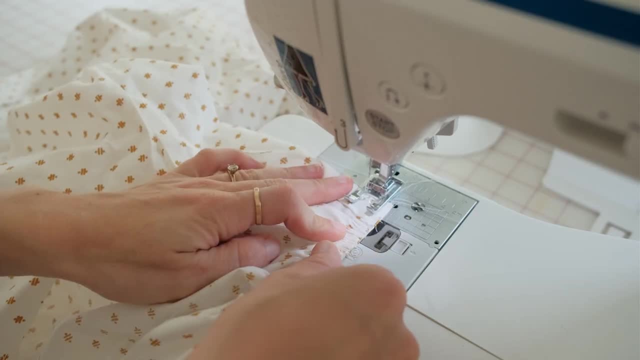 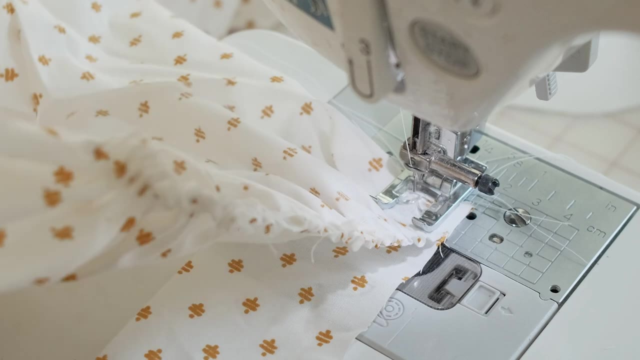 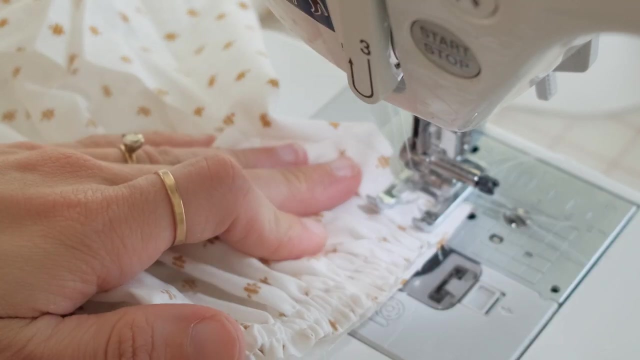 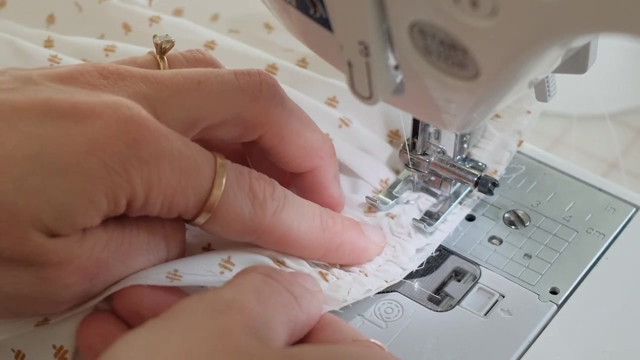 the front gather section and sew across at 1⁄2". Make sure you move the stitch length back to its original state so that it's a tighter stitch and it won't fall out later. Then you're going to turn over your front piece. 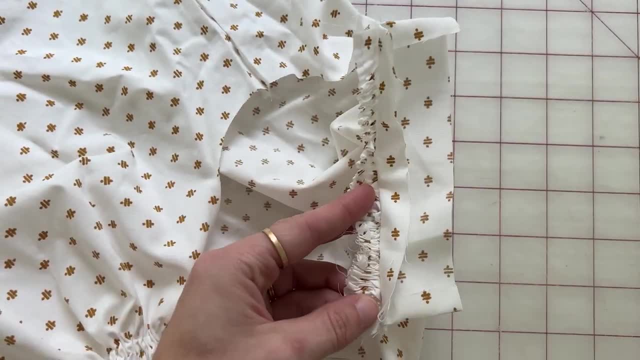 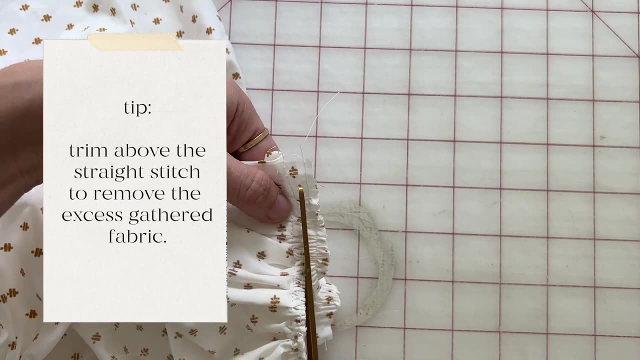 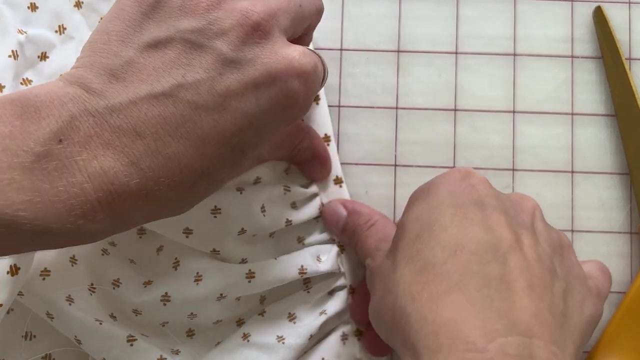 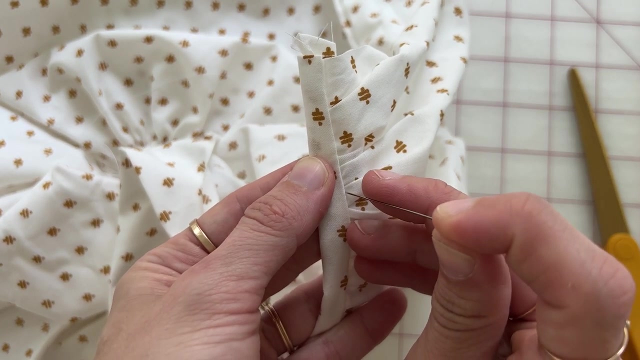 And you're going to fold it and iron, We're going to turn our back over so that we have the same length it, so that you can fold it once more and hide this gather section within this front panel piece. Now that it's all ironed in place, you can poke a pin through where the edge is. 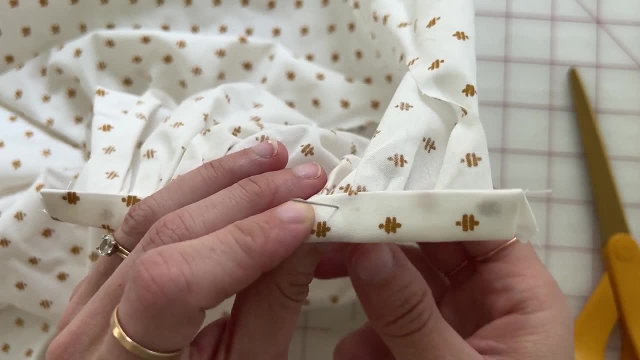 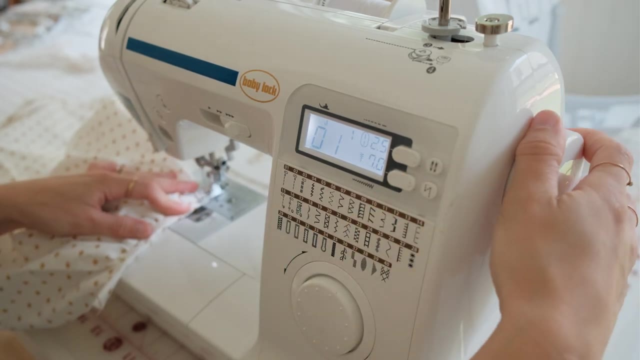 and this will show you if you're gonna match up and catch the piece on the back, so you don't miss it. you want to sew right over this, so if it's a little difficult, you can hand sew this, but what I like to do is just move the needle. 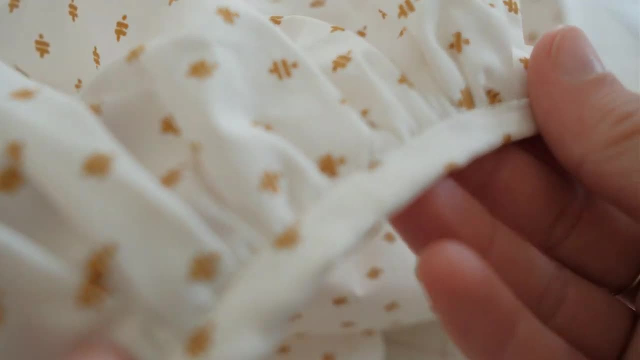 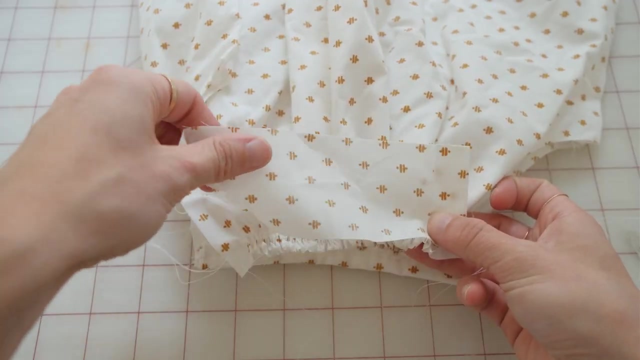 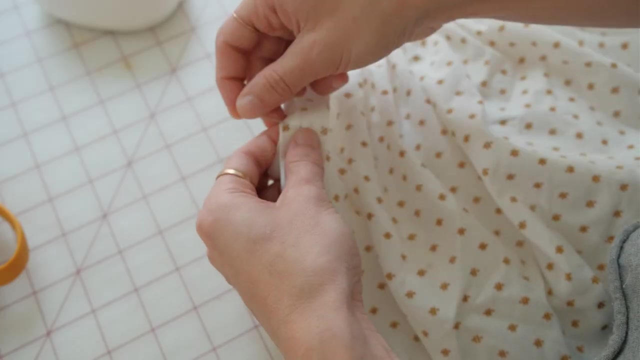 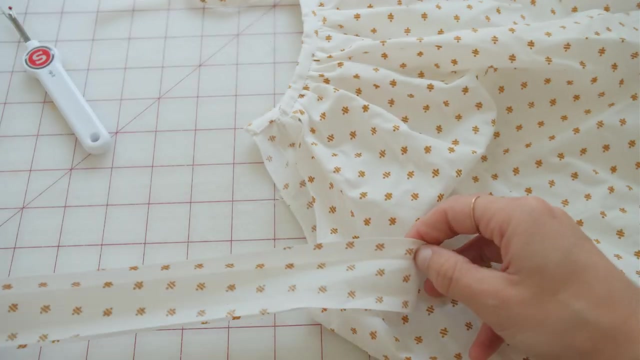 position over to the right, so that it's easy and I know exactly where the needle is gonna go. Then sew across the front and do the same steps for the back. Now for the straps. you're gonna take the bias tape that you already prepared, and 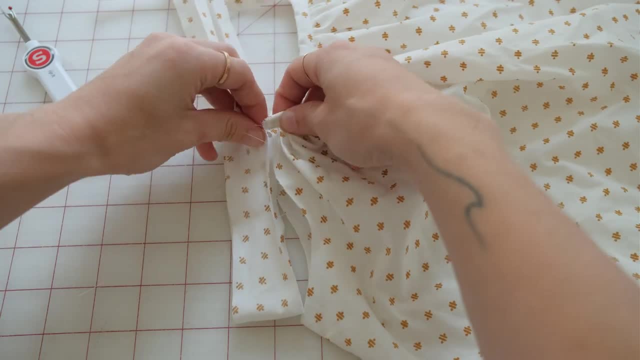 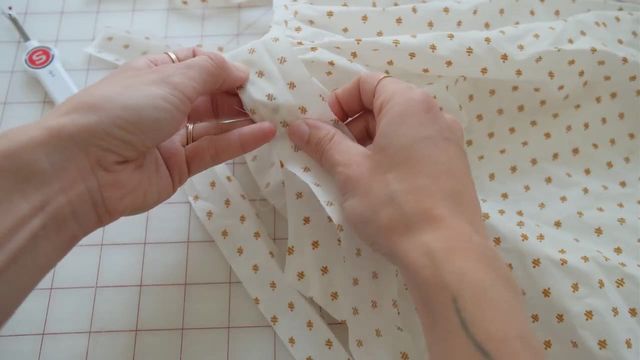 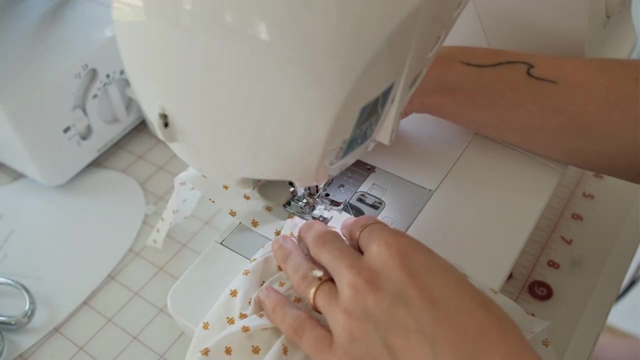 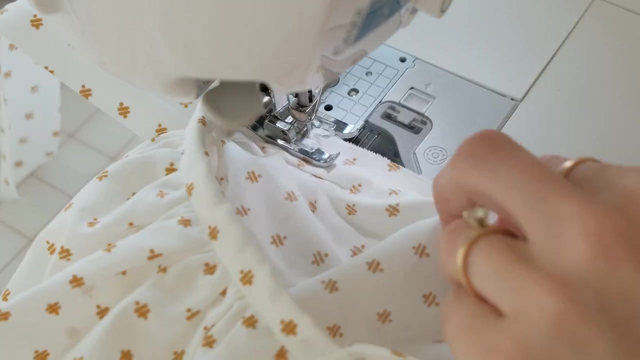 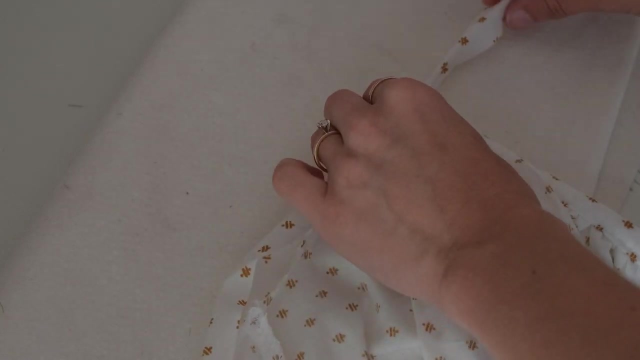 fold it in half, mark the center of the armpit. then you're gonna pin it in place all the way around the armhole and start from the top and sew right sides together. the bias tape to the dress And it's already ironed. so this should be an easy step and you're just gonna. 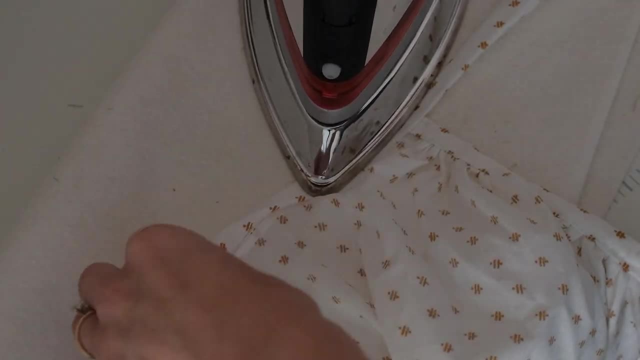 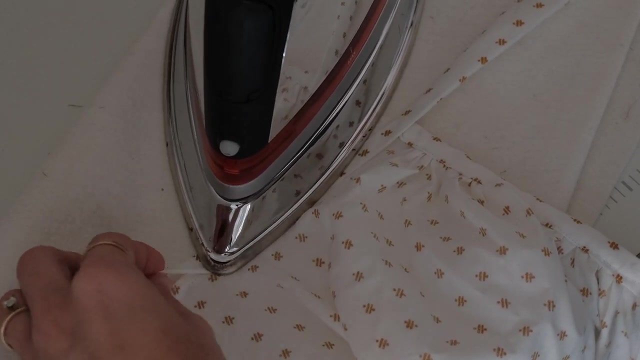 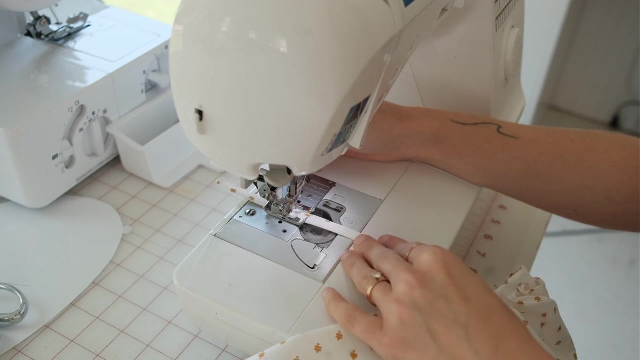 enclose this opening within the bias tape and do the same thing with the pin to make sure that when you sew you're gonna enclose the bias tape and not miss it. So now you can put it under your sewing machine, move the needle over if you need.